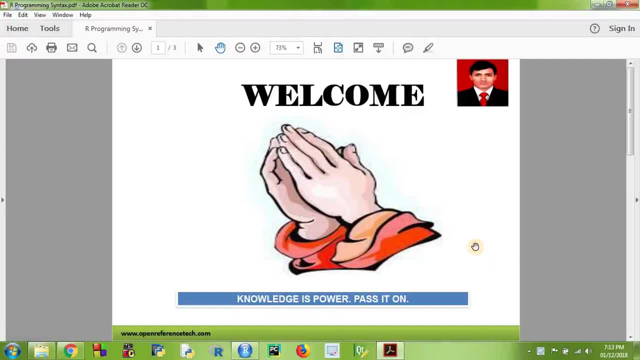 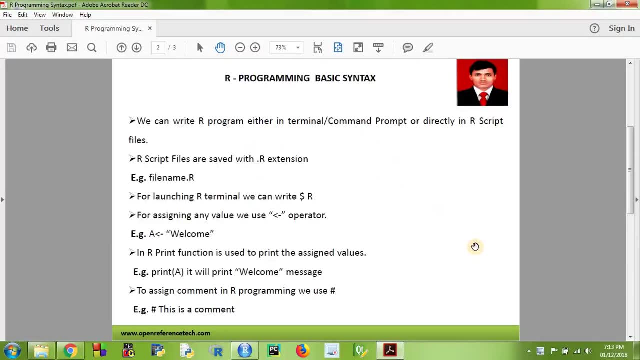 Welcome in this video series of R programming language. In this video we will learn very basic syntax of R programming with some important example. First, we can write R program either in a terminal command form or directly in a R script. files For writing R scripts file. 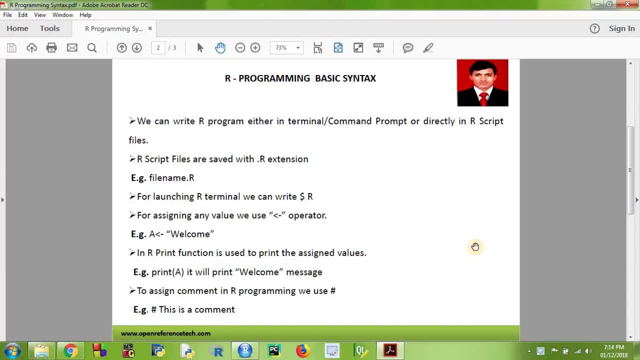 we need to save with R extension, For example Filename- withR For launching r terminal. we can use or we can write capital R on ubuntu terminal. In Windows you can directly click on Exe short- Jetzt garantisi cybersecurity shortcut if you have installed R console on. 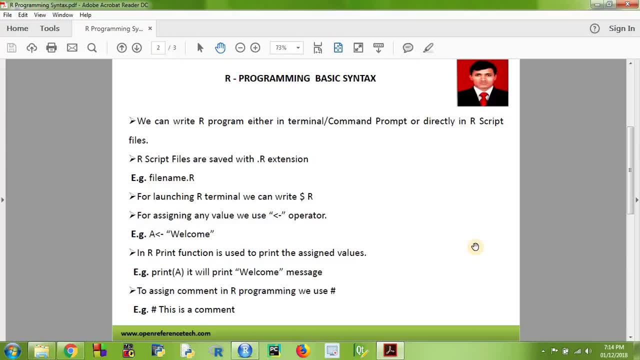 your system For assigning any value. To create a new class from with R extension, you should start with huse berger value. we use assignment operator, which is shown here in this video. Here I am going to assign, for example: here I am going to assign: welcome to A. So this message will. 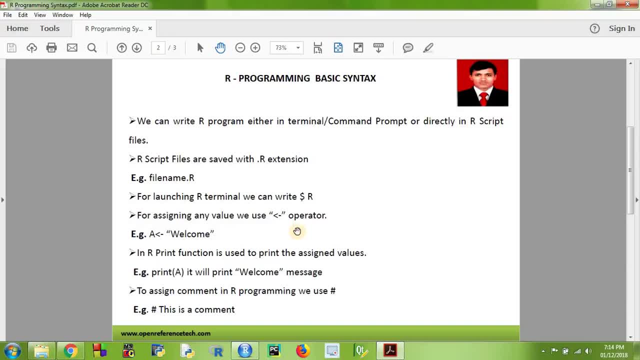 be print. when we are going to use a print function, whatever the value or the message which is assigned a particular variable, For example print A, it will print a welcome message To assign comment. in R programming we use hash function, For example hash- this: 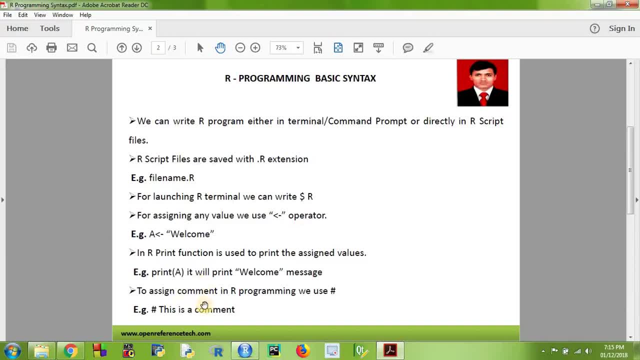 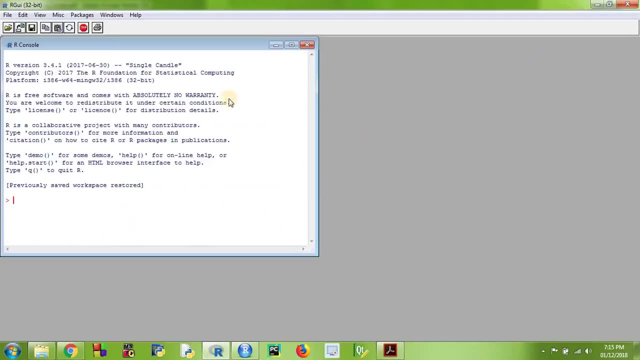 is an comment. Now let's see practical implementation of basic syntax of R programming with some example. First we will go through the R terminal, R console. So this is a R console. Here we can write whatever we have seen in the simple example. 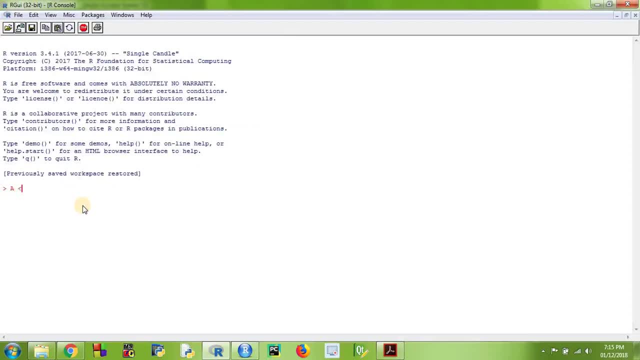 If suppose we have a simple example, we can write whatever we have seen in the simple example. If suppose we have a simple example, we can write whatever we have seen in the simple example. If suppose we have a simple example, we can write whatever we have seen. 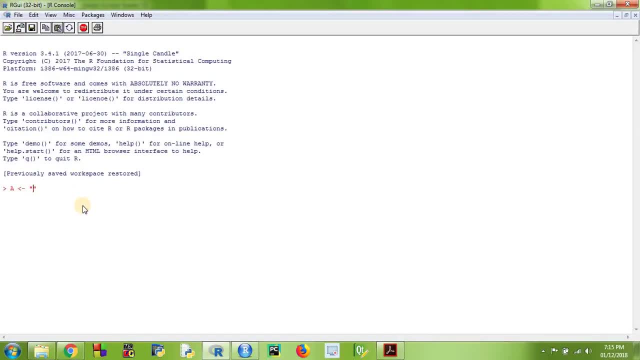 in the simple example, In double quotation, write down the message. whatever you want to print. Now I am going to print a welcome message. Hit the enter So welcome, which is assigned for A. Now you just type here: capital A, So welcome, which is printed now.